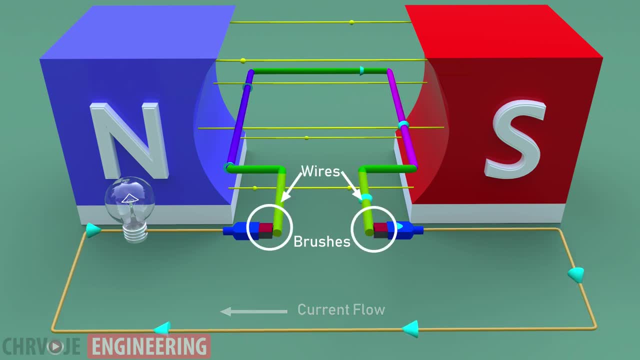 what we require is that these brushes constantly keep changing contacts between these wires for each half of rotation. So if the current flows in this way, in this position, this brush must be connected to this wire. So current flows like this and comes out. 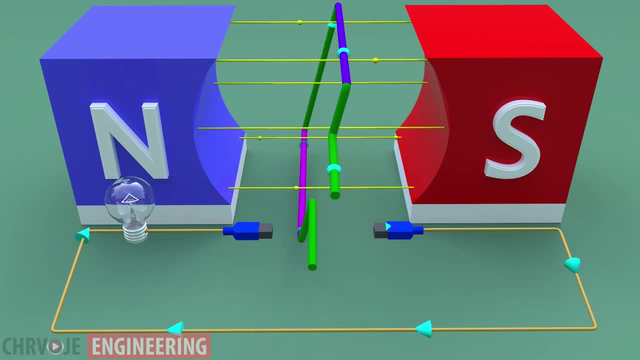 But when the coil rotates you can see that when the coil comes to this position, the direction of the current changes. If we want to keep the current in the same direction, we must this brush to be in contact with this wire Right. 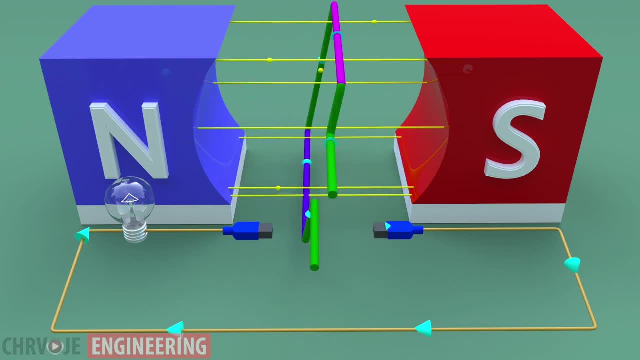 And then again, when the coil comes to this position, again the direction of the current changes, and again we want this brush to come in contact with this wire. Probably we already learned that For every half rotation we must change contacts between brushes and wires. 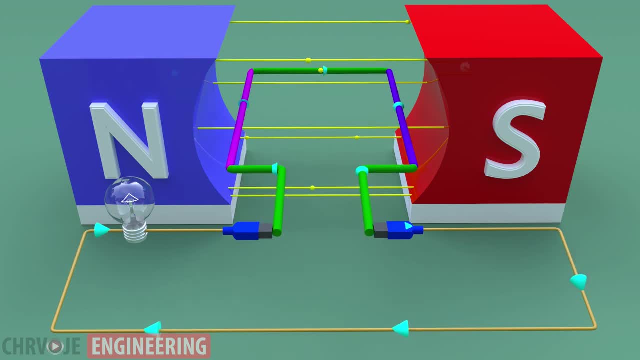 But how do we make this process happen automatically? We can automate this process by adding split rings. Split rings, as the name suggests, is a ring that is split in between giving two half rings with the same gap in between. Now let's see how the split rings automatically change contact for every half a rotation. 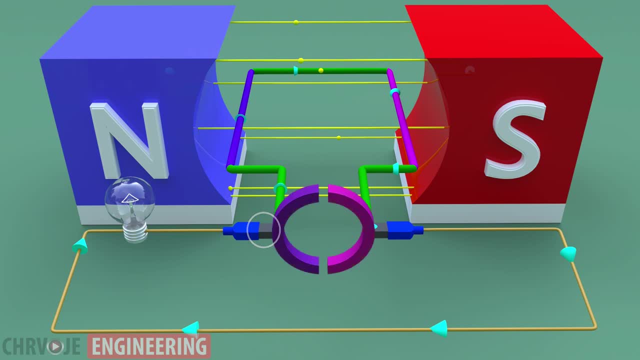 So right now, this brush is in contact with this half part of the split ring: violet color. When the coil rotates and comes to this position- the direction of the current changes- and this brush now is in contact with the other half part of the split ring: pink color. 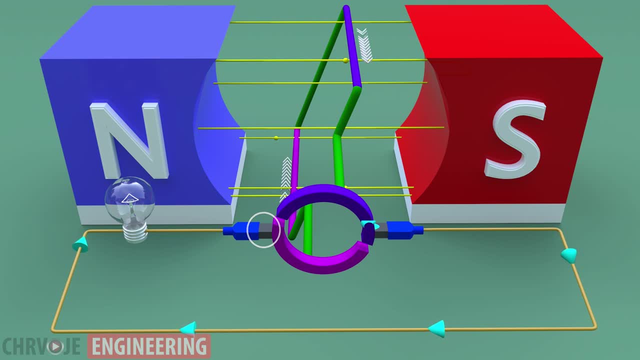 This arrangement provides that current flows in the same direction Again as the coil comes to this position, finishing another half a rotation. you can see that this has only changed. contact Brush is in contact again with the violet color half part of split ring. 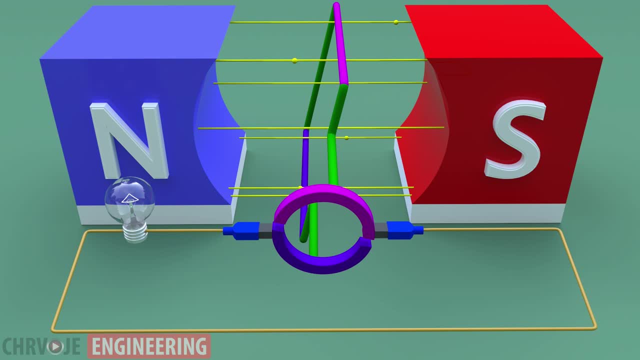 In this way the DC generator is built, where the current only flows in one direction through any external circuit, and in this arrangement with brushes and split rings, which helps us to automatically change contacts. we call them commutators, So split rings act like commutators. 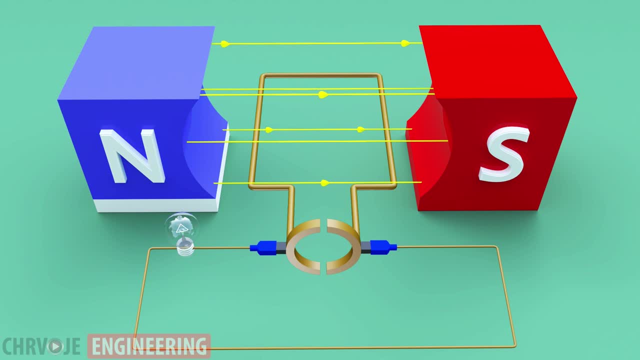 The next thing we must mention, that it's really important for working principle of DC generator, is: how can we determine the direction of the current magnetic field and force? To determine all this we must use Fleming's right hand rule. So we will explain how can we use Fleming's right hand rule. 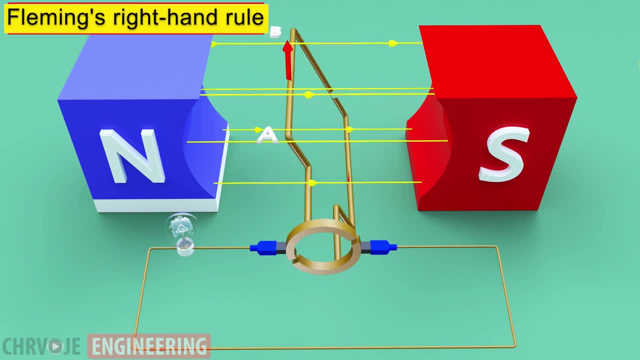 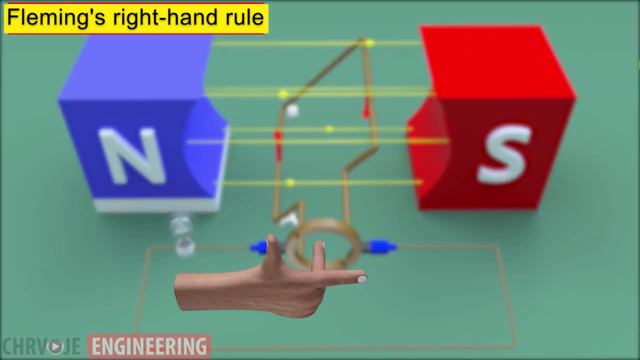 As you can see, the rotation of the coil is clockwise and the force acting on part of the coil aids the rotation Similarly B, pushing that part of the coil upwards. So to know the direction of the induced current, we apply the Fleming's right hand rule. 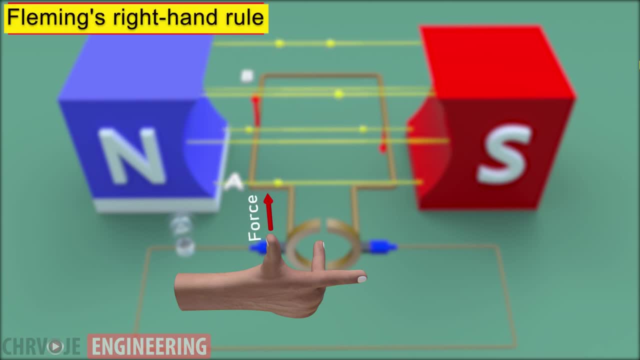 How do we do that? We place our right hand so that the thumb points up showing the direction of the force. The index finger or the finger pointing in direction of the magnetic field from north to south pole, and middle finger will point in the direction of the induced current. 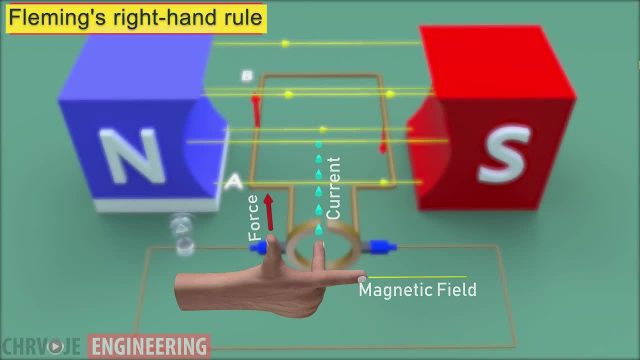 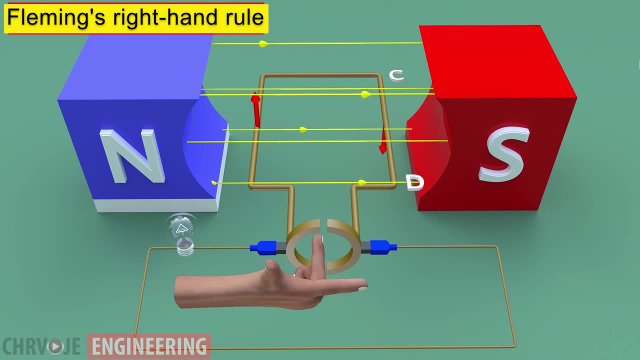 which is in our case from A to B. Similarly, to find the induced current in a part of the coil CD, we again use Fleming's right hand rule. So the rotation of the coil is clockwise and the force acting on part of the coil CD. 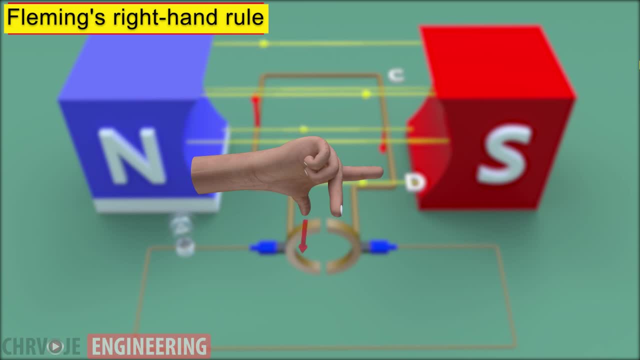 pushing that part of the coil downwards. The thumb points down indicating the direction of the force indexed finger, or for the finger pointing in direction of the magnetic field from north to south, and the middle finger will point in the direction of the induced current. 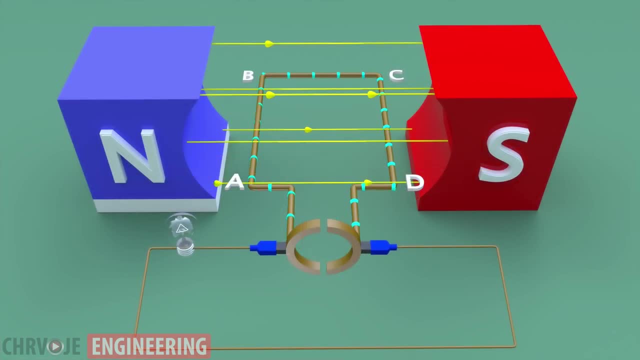 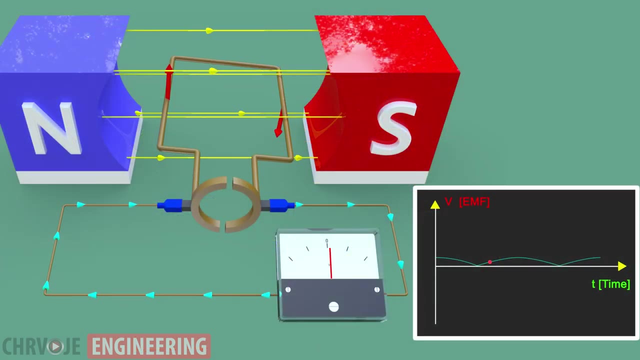 which is in this case from C to D. So, to conclude, the induced current follows the path ABCD of the coil. The effect of the split ring commutator in DC generators is to ensure that the induced EMF is always in one direction. 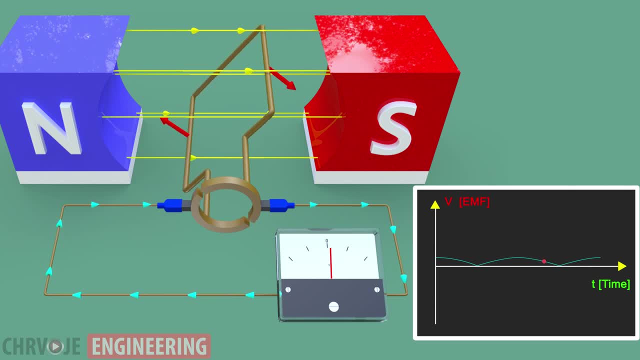 We can see that in this graph, where V represents the amount of induced EMF and T represents time. You will notice in the graph how the sine wave changes with rotational speed of the coil. The coil, in this case, has clockwise rotation. Increased rotational speed of the coil increases the amount of induced EMF. 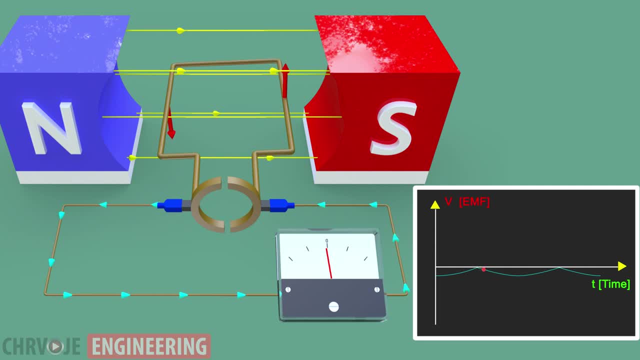 the induced EMF has a positive sign. Also, you see the example how the sine wave changes with rotational speed of the coil. when the coil is rotating counterclockwise. Again, the increased rotational speed of the coil increases the amount of induced EMF.